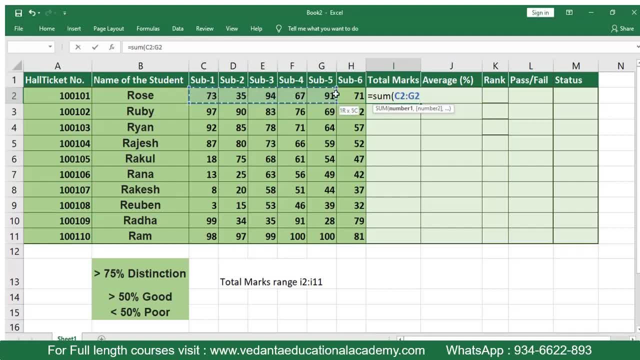 subject one that is C2, and it will just drag down to the last subject, that is H2, and directly close the bracket and press enter- And here the total marks of the student rose is a 431- and simply select the cell and click on the dragger handler. So when you move up on the cell you will get a plus sign in the 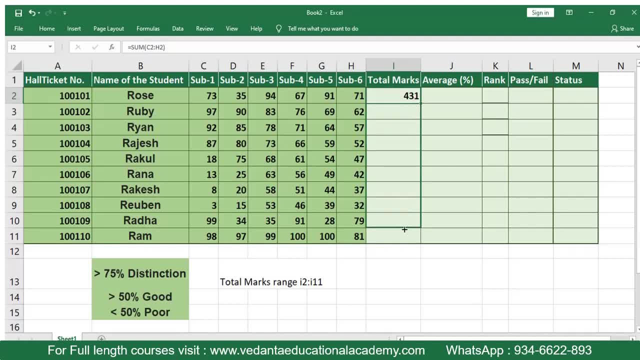 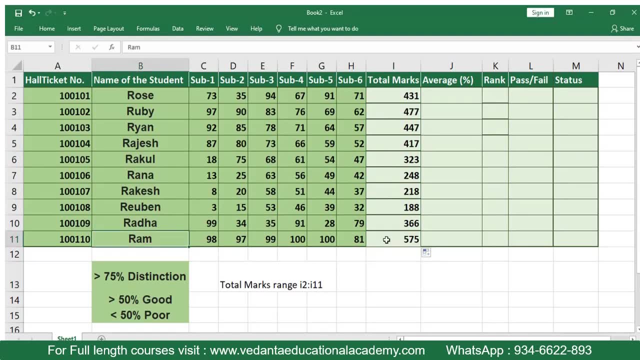 black color. So just simply hold on and just drag down. Yes, So either. so your Mr Ram is the person who is getting the highest marks out of 600. He is he is he secured a 500 and a 700.. Next year I would like to get the, the average marks of the student. So simply equals to. 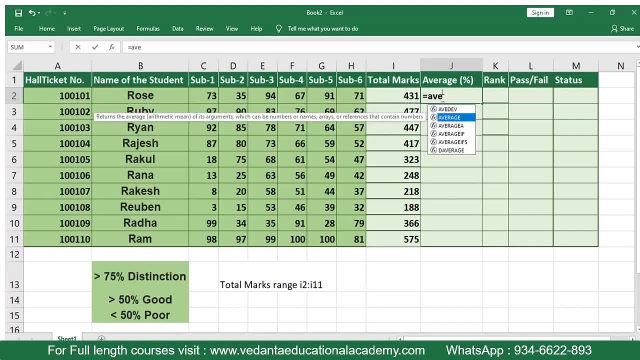 equals to average, equals to average and simply select from subject one to subject six and directly close the bracket and press enter, and average is 71.83. or else you also can do directly equals to select total marks And here you have the total of subjects six and the same: 71.83 is simply this drag down. 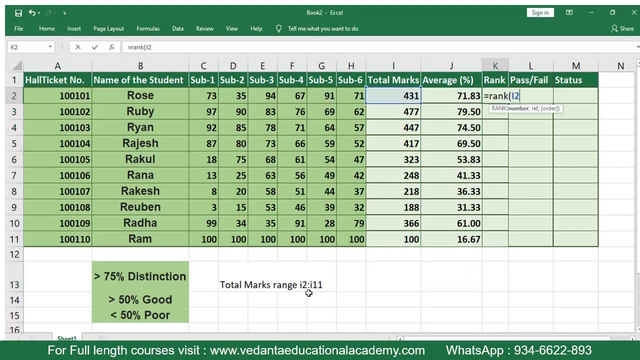 And here the marks, here the average of this student. Nice, simple, equals to rank open bracket. I would have to compare the marks. rank of 431, that means I 2, comma in the range. what is the range address? I 2 to I 11.. Then you just 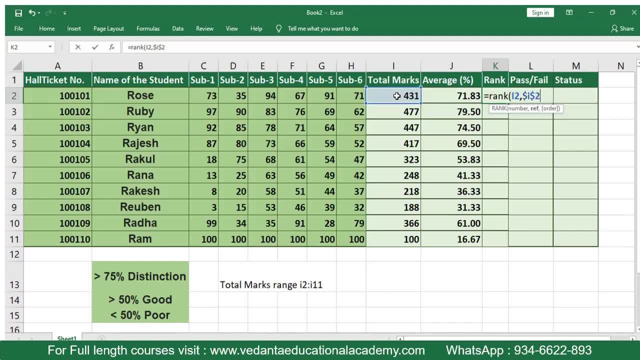 simply enter a dollar I dollar 2, colon. Just before that you suggest add dollar sign to 5.. So I press enter dollar sign to fix a standard input range: i22. that means dollar i dollar 2, till where again i11. if the address is i11, then you enter dollar i dollar 11, then simply close, then press enter. 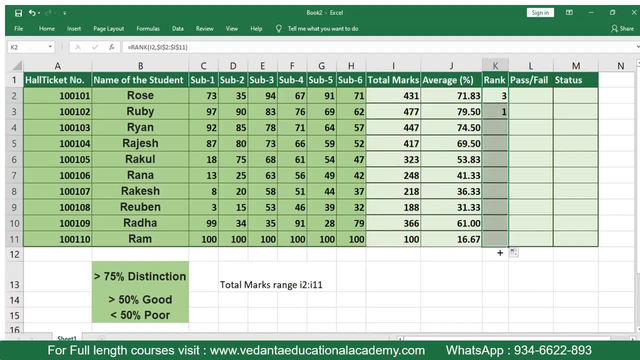 then now, this time, if you once drag down to still last cell, even in the last cell also, it is taking a standard inputs. so this is how it works, and here i just change it manually. so i'll do one thing, i'll just drag it down. yes, now this person is getting a 600 marks, so the person is awarded. 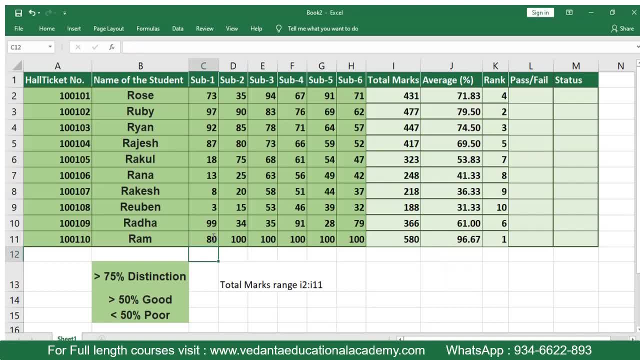 to rank number one if i change anything here and again. 80 gain, 80, 80, 80, 80. okay, so the person is getting the highest marks of 480, so don't worry, i'll be changing. uh, here i'll just keep it zero now. this time you can see that the person has awarded as fifth rank and the person who 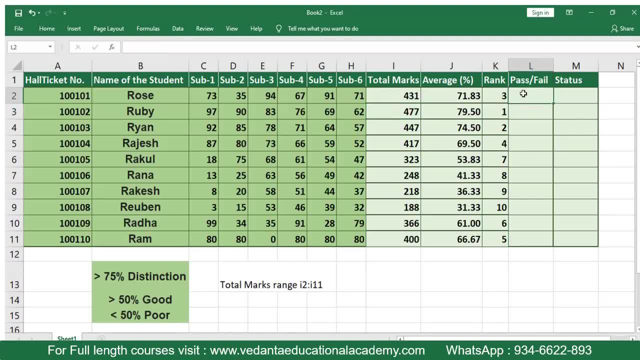 is getting. 477 is the highest marks, right. so next we will understand that: how to calculate pass or fail and what is the condition. the student should get greater than or equals to 35 in each subject will be given a status as pass or as fail, is it correct? so now we need to compare each subject. 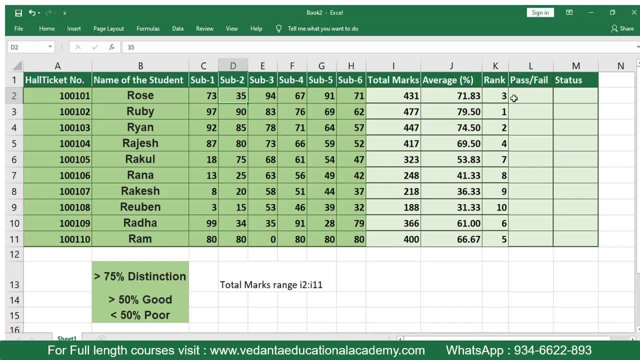 right. so here we cannot compare. if by using if function we can compare, by using if function we can compare, we can perform only one logical test, correct? if you like to perform multiple logical tests, that means see if you're using only if, for example, only subject one, if c2, that means subject one, is greater than. 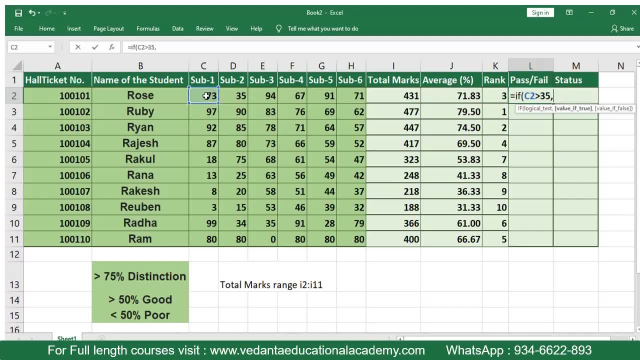 35 comma. if the value is true, pass or else fail. so you can, by, by using if formula you can, you can. you can perform only one logical test, the here, whether they are pass or fail. but now these time you like to compare total six test, because the person should get greater than or equal to 35 in each subject. that 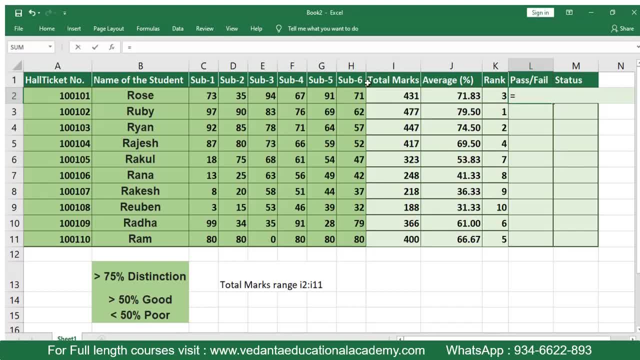 means number of six subjects. so here we should perform six logical tests. so we cannot use a single if formula. so we're going to add equals to if, again equals to if open bracket and then open bracket. so i and help you to add multiple logical tests. so equals to if open bracket and what is the first logical test subject: 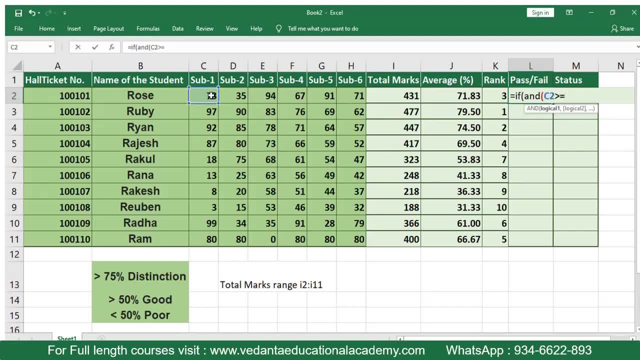 one and greater than or equals to 35 comma. what is the logical test to? what is logical test to? again: subject to greater than or equals to 35 comma. logical test for logical test 3: select this subject, that's e2. that means subject 3: greater than or equal to 35 comma. again subject 4: greater than or: 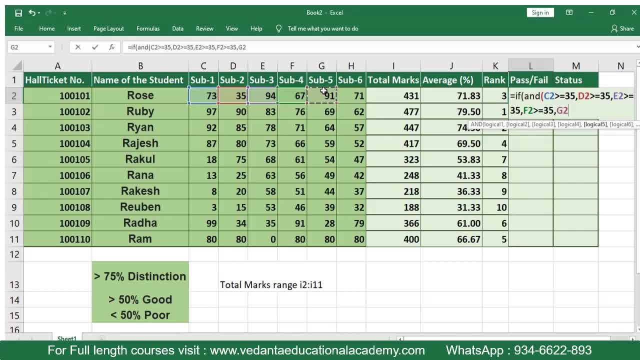 equal to 35 comma. subject: 5 greater than or equal to 35 comma. the last logical test, that is the sixth logical test, that is h2 greater than or equal to 35. now it is done right, then simply close the bracket comma. so in all these subjects, if c2 is greater than equal to 35, d2 greater than 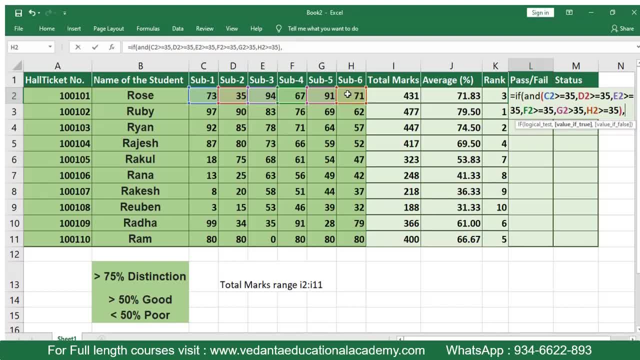 equal to 35 in all subjects. if the person is getting greater than or equals to 35, then the person will be given as the result: double comma open because they're going to add a test. double comma open, p a s s pass. double comma- close comma, if it is, if any of the logical test is not given. 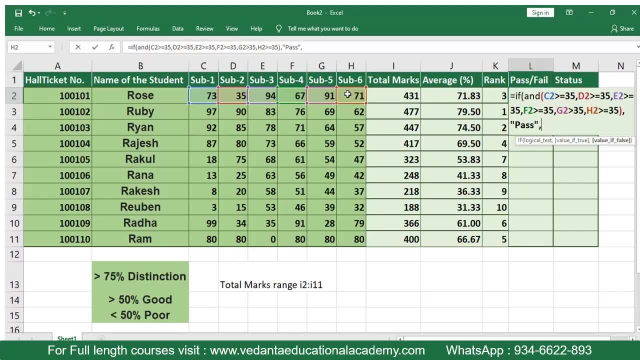 is dissatisfied, then i would like to. it will become as a false, false statement. so i would have to print as f, a, i, l, double comma, close, then close the bracket. so how simple, it didn't directly press enter. so so here the person in all subjects is getting greater than or equal to 35, so the person 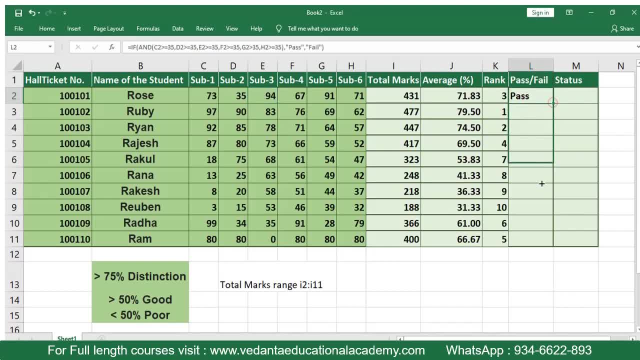 given the statement as fast, then simply drag it down, that's it. and here you can see that all these students are having pay failed because they're getting 18 and he's getting 18 and he's getting 13 here. if i change, if i change these marks to 35 automatically, the student state has been. 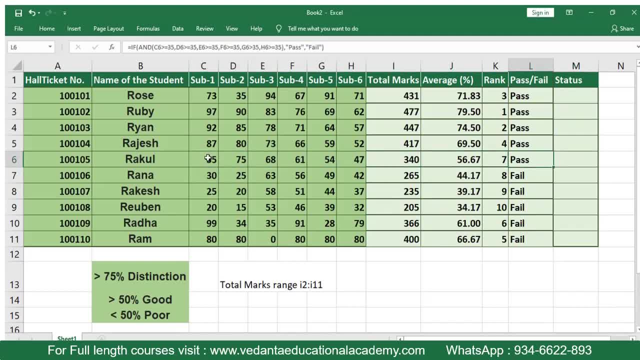 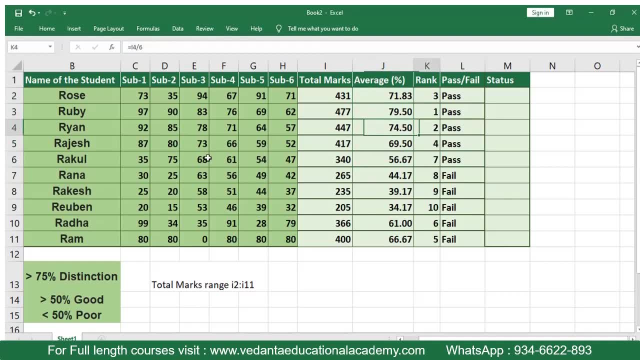 changed from fail to pass is correct and next we'll be using the status of whether they are getting a distinction. marks are good, yeah, poor. that based on the a percentage right, so they're simply equals to. equals to if open bracket. equals to if open bracket. what is the logical test if the 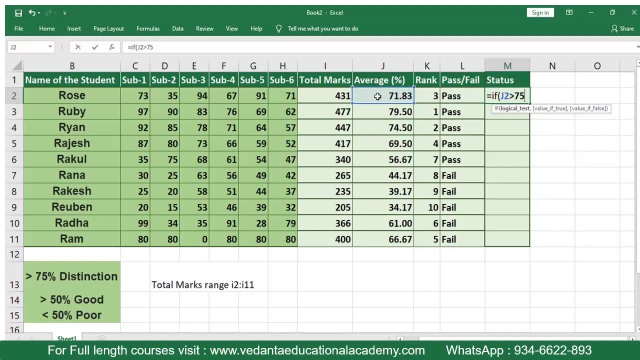 person is greater than or equal to 75. so target is greater than or equal to 75. so that is the question: what is the logical test? i can say that the question is: what is the logical test? so target is greater than or equal to 75 comma, double comma, open distinction. 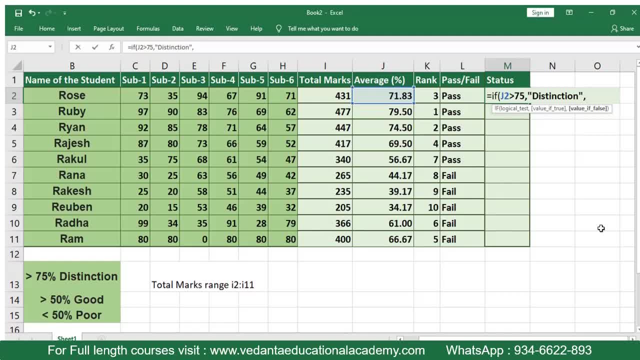 double comma, close comma. i'm not here. here the system is asking value if false. but here i'm going to add one more if, because it means we are going to add a. the if is known as nested if. right, so i'm going to. instead of giving false again, i'm starting if. 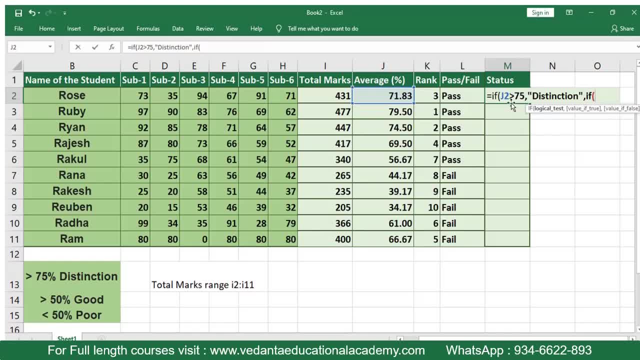 again. if, if j2 is greater than 35, distinction again. if j2 is greater than 50, double comma, open, double comma, open comma. uh, if it is more than 50, then i would like to show as good, because good comma. if, if it is not more than 75, then it goes for whether if it is, if it is not, 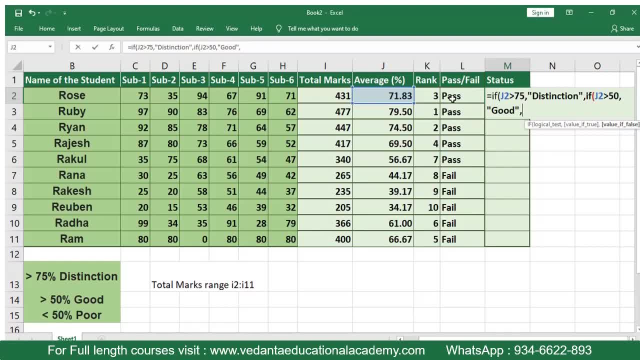 see first system understand to calculate whether the this j2 is more than 35 or not. if it is more than 35, directly shows the. shows the result as distinction. if it is not more than 75, then it is going to jump to calculate whether it is more than 50. if it is more than 50, it is going to show the. 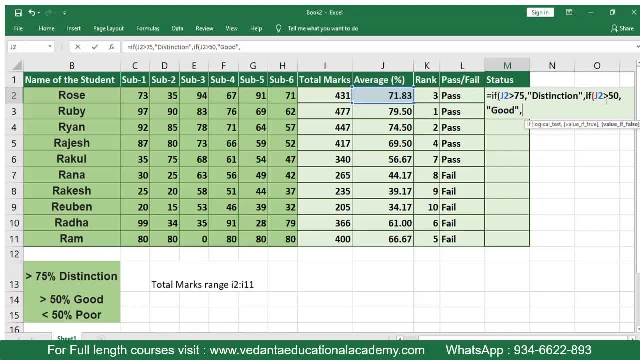 show the result as good. if the both, if the both tests are failed, that means it is less than less than a 50. then i would like to show as: uh, what is that? it's poor, right, poor. then double comma, close, close the bracket, then press enter. maybe i, yes, i need to see here i have one bracket is open, again one more bracket. 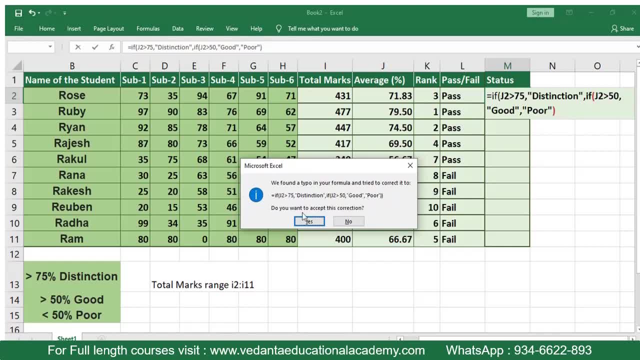 is open, so we need to close it two times. so here the system is going to show the same thing, but you want to accept the correction? yes, of course. yes, here the system is going to show the same thing, but you want to accept the correction? yes, of course. 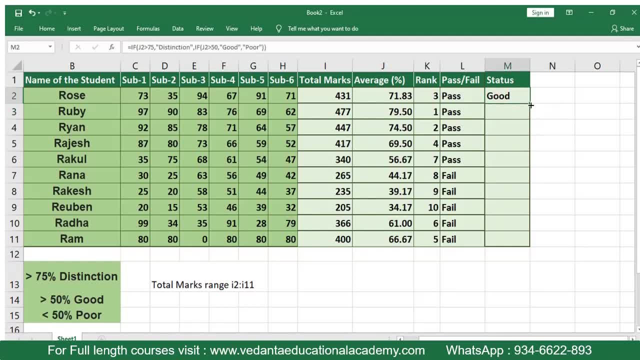 system added one more bracket, don't worry so, simply just drag it down. yes, automatically, all the student data has been converted. if you want to make any changes in this, automatically all the data will get changed: the 90, 90, 90 now. still the student is showing the status as failed because